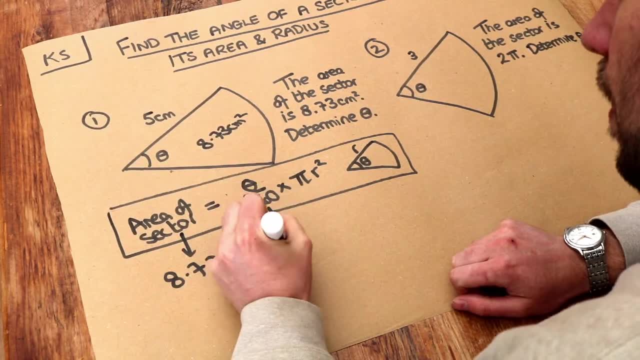 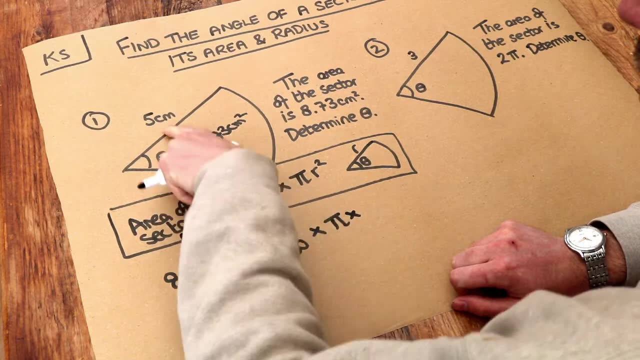 well, theta over 360, well, the theta here, we don't know. we'll leave it as theta and then we're timesing by pi times and then r squared so r here is five, so pi lots of five squared pi times. 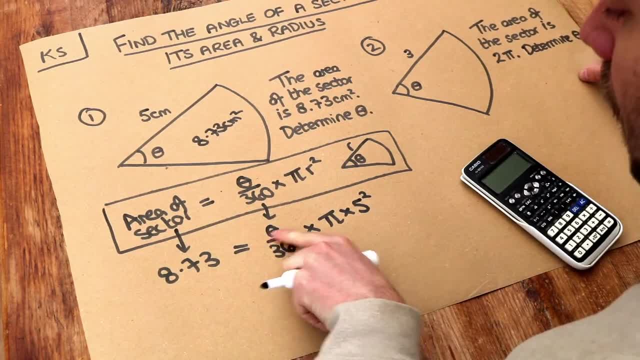 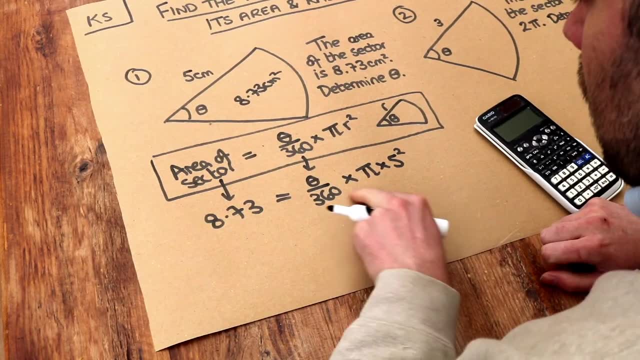 five squared. Now, this is an equation in terms of theta that we need to solve, so we need to find out what the value of theta is. so let's try and gradually get rid of the various things around theta. Well, I might first be tempted to divide both sides of the equation by this pi and the five. 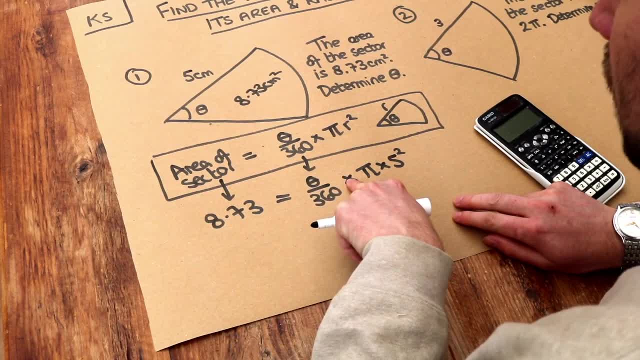 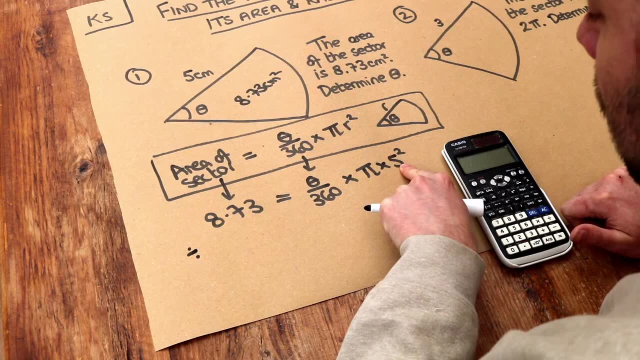 squared, because the theta is first divided by 360, then you times it by pi and five squared. so we're going to divide both sides by the pi and the five squared. well, five squared is 25, so we're dividing by 25 pi. 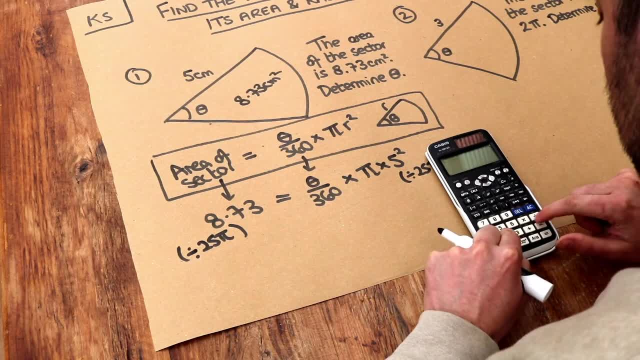 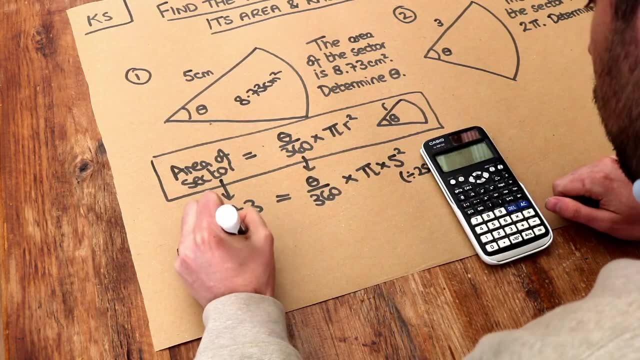 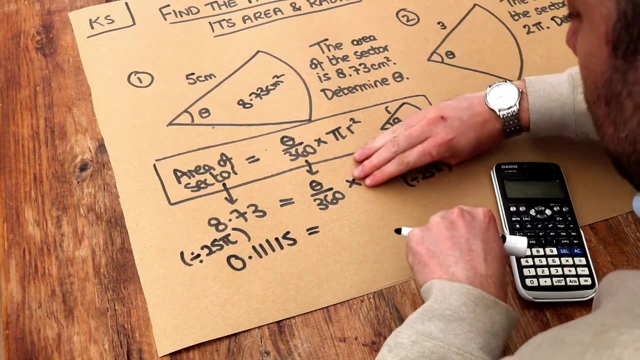 So we do 8.73 divided by then I put in brackets 25 pi, just to be on the safe side, and that gives you 0.11115.. That's got rid of the times by the pi and the five squared the 25 pi, leaving just. 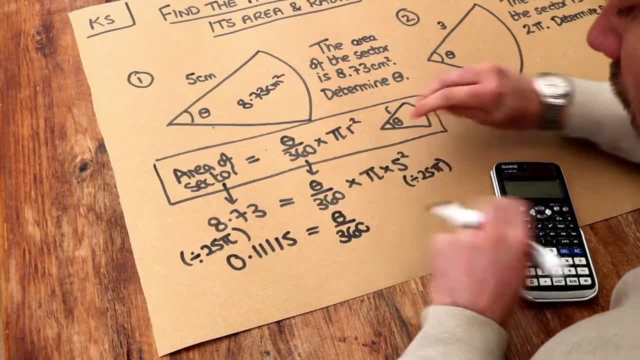 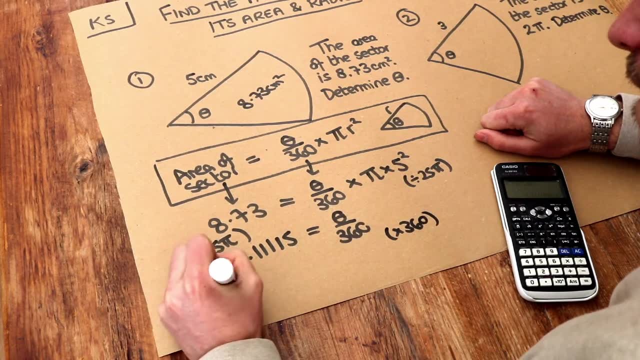 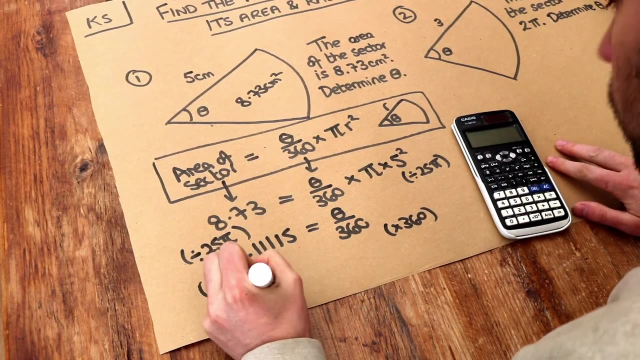 theta over 360.. Now, if theta's been divided by 360, how do you get rid of that over 360? Well, you times both sides by 360. So our value here: we times it by 360 and that gives us 40.02, or, to just three significant figures, 40.0. 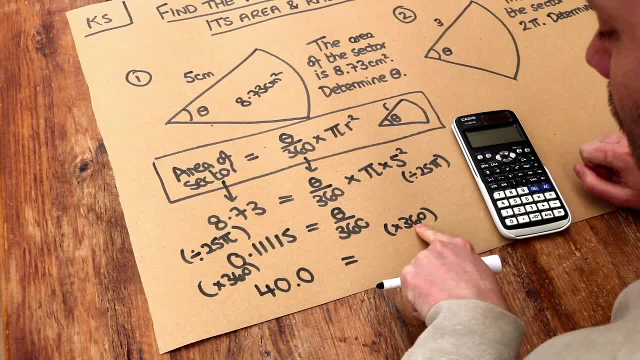 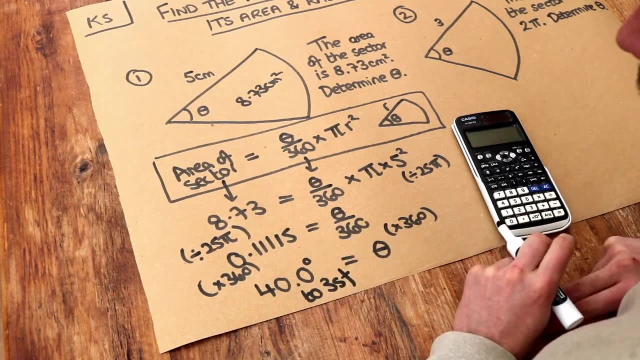 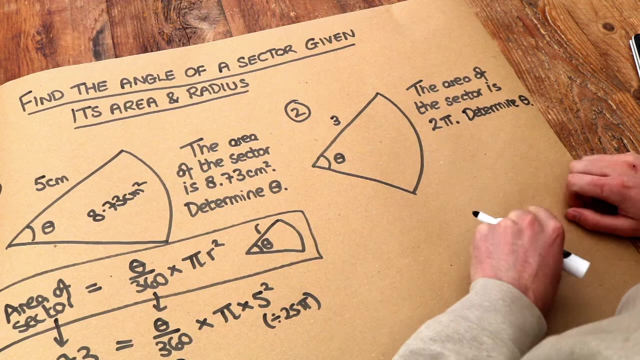 And that is theta, because the times by 360 gets rid of the over 360 and it's in degrees. And this is two, three significant figures which we should state, and that's the final answer. Let's do it with the second one. here, The area of the sector is two pi. now it's given us the area of the sector in terms of pi. this 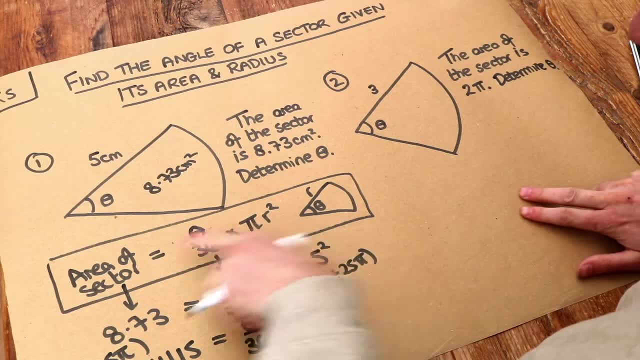 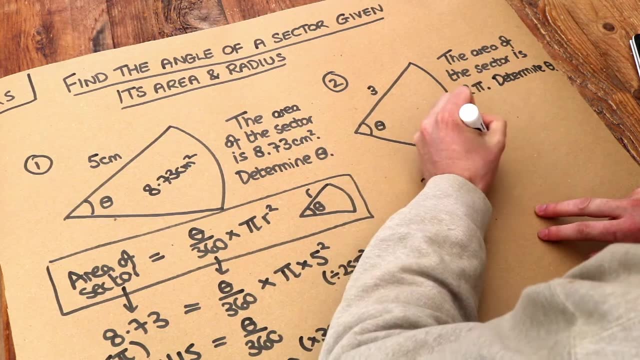 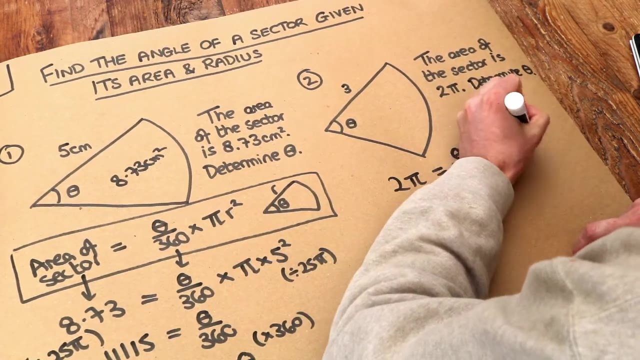 time determined theta, We would do exactly the same as we did before. The area of the sector which is two pi is equal to theta over 360, theta over 360, times by pi r squared. so pi times three squared, Let's just. 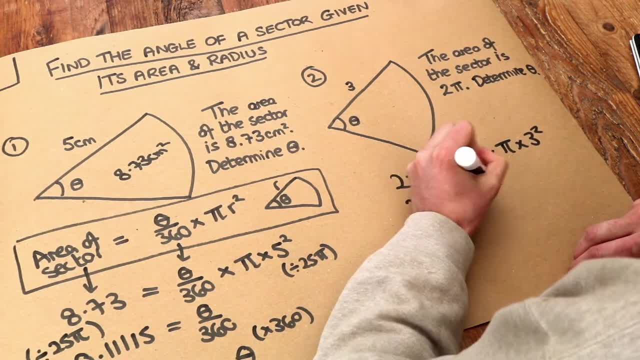 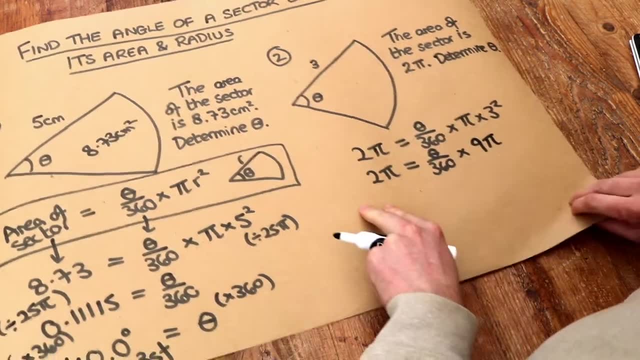 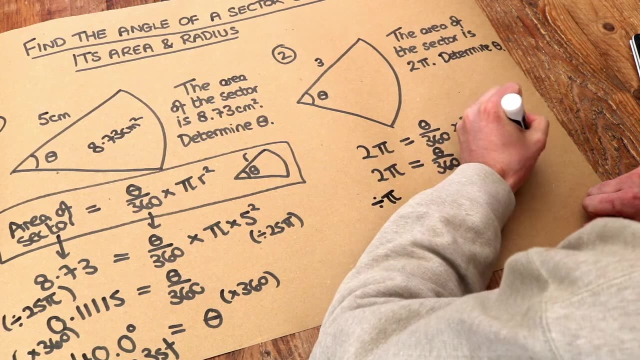 tidy this up a bit first, unlike before. So pi times three squared, that's nine times pi. we just write nine pi here. So what could we divide both sides of the equation by? Well, let's just divide it just by pi, this time first.